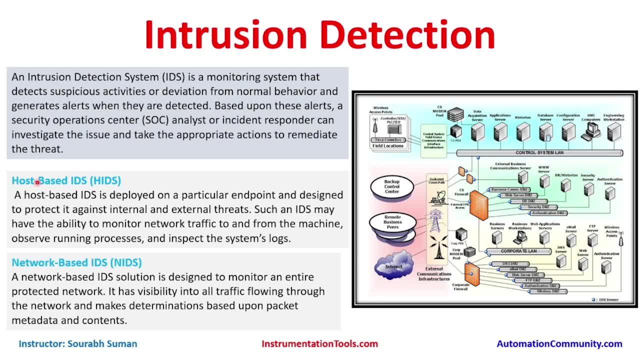 us suppose if a computer is there on that you can install, implement this host based ideas, It will check all the files, it will check all the processes, whatever is running, what type of activity these processes are doing, If there are some communication going on that host, if there. 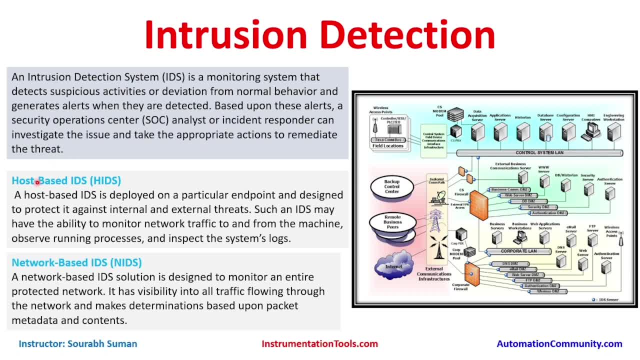 is a communication happening between the application and system software application and the network. those all type of communication will be tracked, and from the machine only, and will inspect system logs And in case of any deviation from the baseline behavior it will initiate an alert. Another type is the network based ideas. So a network based ideas solution is designed to 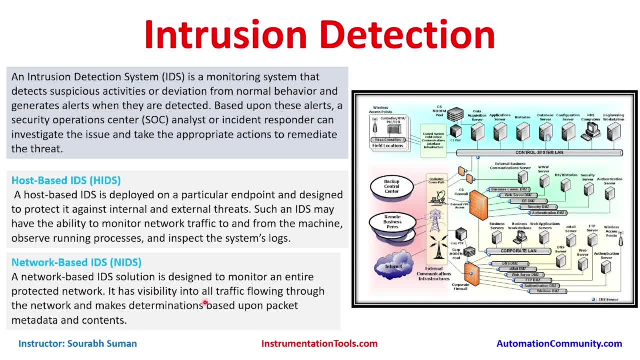 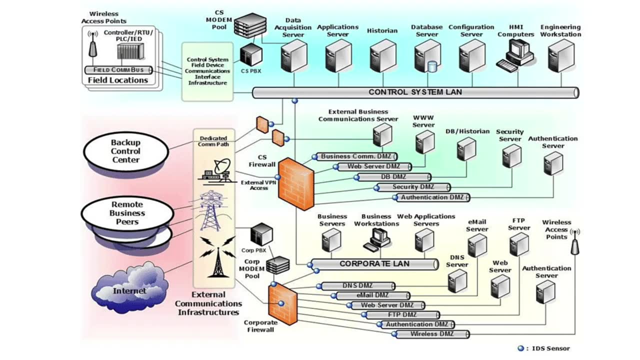 monitor an entire protected network. So it has visibility into all traffic flowing through the network and makes determination based upon the packet metadata and content. So it will capture all the network traffic. like you have seen here Earlier we discussed this network architecture, So all these dots are the ideas sensors. So this will pick up all the communications. 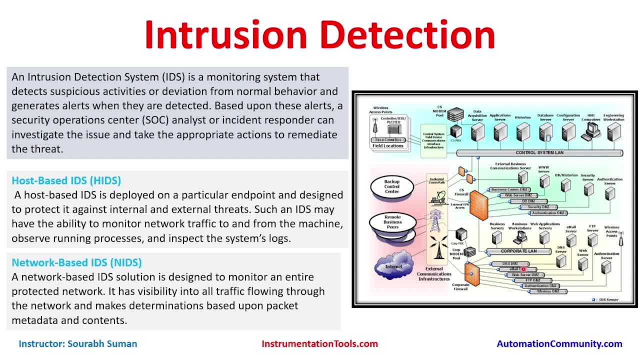 whatever happening between. let us suppose if we take this one, so email server to, it is going to external communication infrastructure. So whatever communication will happen through this complete network capture will go to these ideas and then it will analyze what type of traffic is flowing. 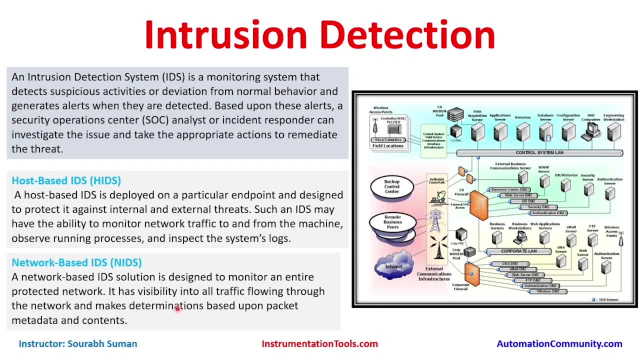 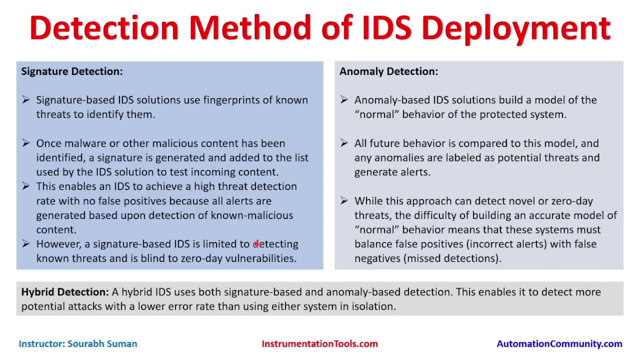 what is the data inside that traffic, how this communication can be a one liberty or can be a exploit to our system. So that will be found based on the signatures or based on the created rules. So there are some detection methods of ideas also, like I said, that it can detect based on the signature also. So there are basically three modes. 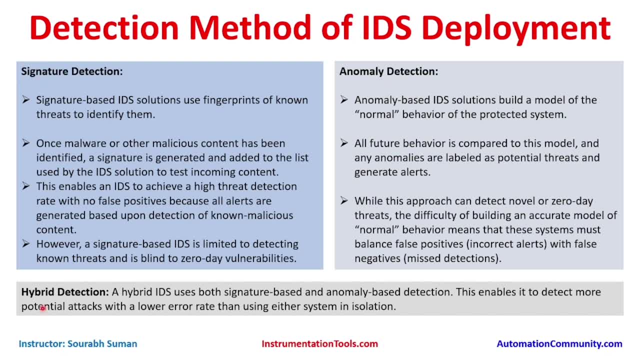 of detection. One is signature detection, another is anomaly detection and third is hybrid detection. So signature based ideas, solutions, uses fingerprints, threats to identify them. so if there is already a some known malware, so it will keep a signature of that malware and once malware or other malicious content 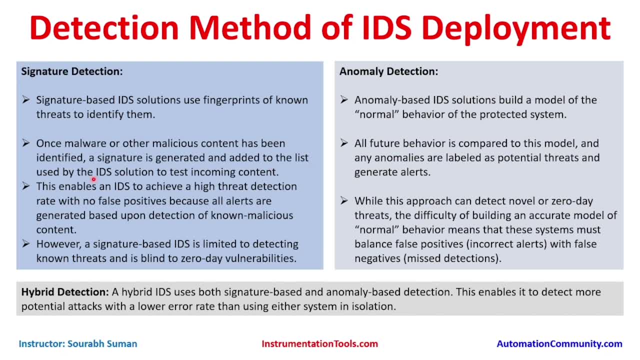 has been identified, a signature is generated and added to the list used by the IDS solutions to test incoming content. so this enables an IDS to achieve a high threat detection rate with no false positives, because this is just a direct comparison. like antivirus does, so similar for for malwares also. 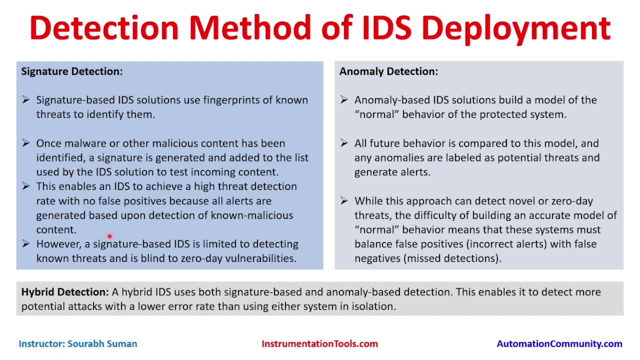 because all the alerts are generated based on the detection of known malicious content. so already it is known. it's not a zero-day attack, so it can find those signatures quickly. however, the signature based IDS is limited to detecting known threats, is blind to zero-day vulnerabilities. so what? 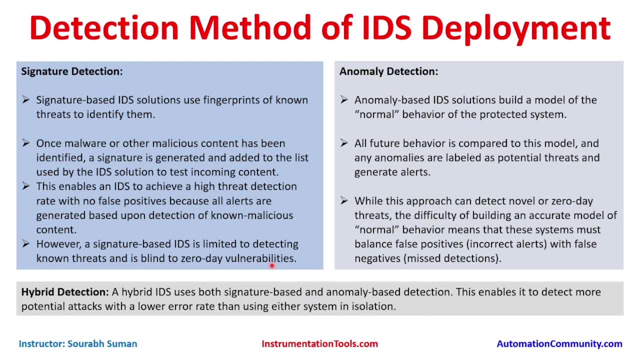 is zero-day vulnerability. zero-day vulnerability is that some malware, ransomware or virus on the internet or threat on the internet which has not been exploited or which has not been in the network prior to this. so that is a zero-day. so it means like is the zero day of that. 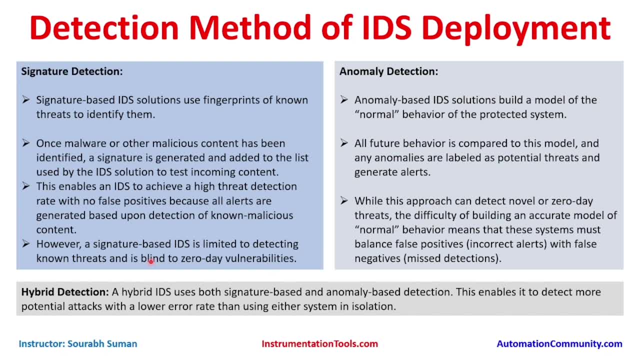 you malware on the internet or for that system. so there is no any known signature of level for that malware. so that is called a zero-day attack. and those are very costly and can be created with very high, huge resource and use compute capabilities and also technical skills. so that is called signature. 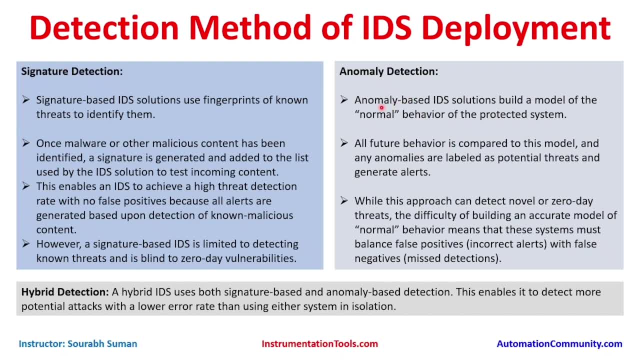 detection. now coming to the anomaly based detection. anomaly based IDS solutions build a model of normal behavior of the protected system. so it builds an model of the normal behavior of the protected system. so it builds an model of the normal behavior of the protected system. so it builds an model of the normal. 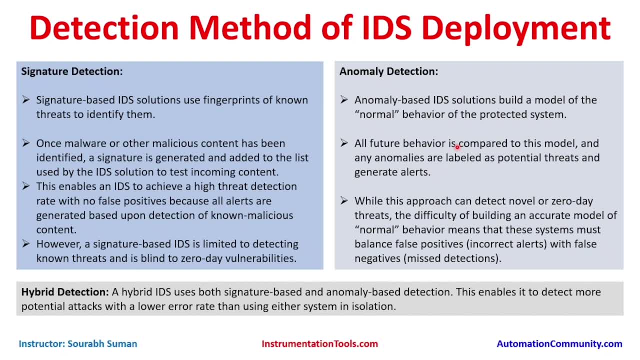 behavior of the protected system. all future behavior is compared to this behavior of the protected system. all future behavior is compared to this behavior of the protected system. all future behavior is compared to this model and any anomaly are labeled as model and any anomaly are labeled as model and any anomaly are labeled as potential threats and generator. so it is. 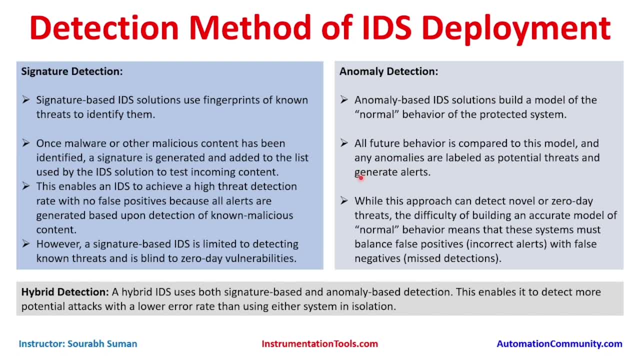 potential threats and generator. so it is potential threats and generator. so it is based on: like machine learning and AI. based on like machine learning and AI, based on like machine learning and AI algorithms, so it will create a model and algorithms. so it will create a model and. 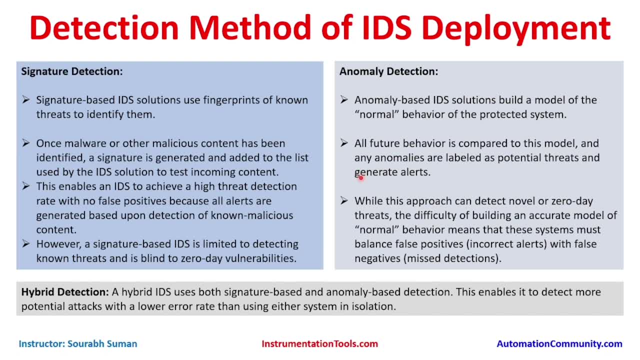 algorithms. so it will create a model and it will baseline your system as per the. it will baseline your system as per the. it will baseline your system as per the current normal operating system, and then current normal operating system, and then current normal operating system and then, if any deviation happen in the behavior of 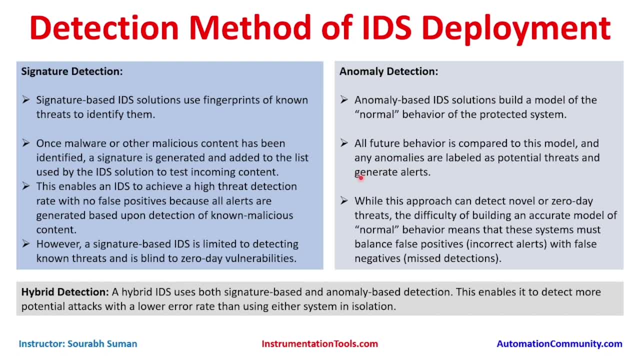 if any deviation happen in the behavior of, if any deviation happen in the behavior of some traffic or some file or some some traffic or some file or some some traffic or some file or some process, it will, it will find the process. it will, it will find the. 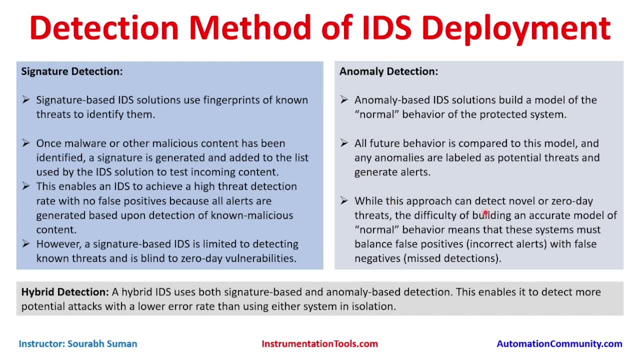 process. it will. it will find the potential threats and generate candidate potential threats and generate candidate potential threats and generate candidate alert. while this approach can detect alert, while this approach can detect alert, while this approach can detect novel or zero-day threats, the difficulty, novel or zero-day threats: the difficulty. 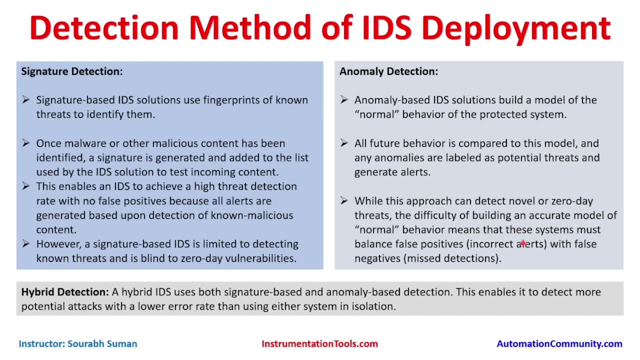 novel or zero-day threats. the difficulty of building an accurate model of normal, of building an accurate model of normal, of building an accurate model of normal behavior means that the system must behavior, means that the system must behavior, means that the system must balance false positive. false positive is. 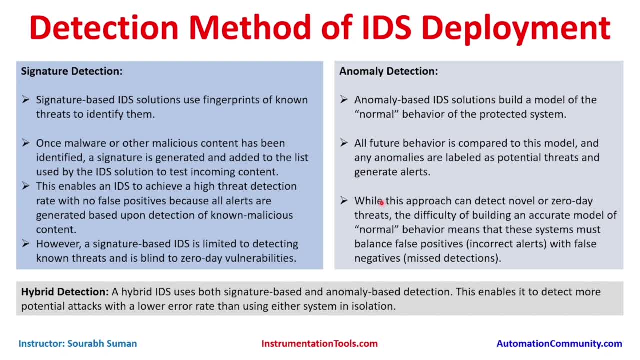 balance. false positive, false positive is balance. false positive, false positive is incorrect error and false negative incorrect error and false negative, incorrect error and false negative misdetections. so this system is now misdetections. so this system is now misdetections. so this system is now maturing and say enough, mature now. so 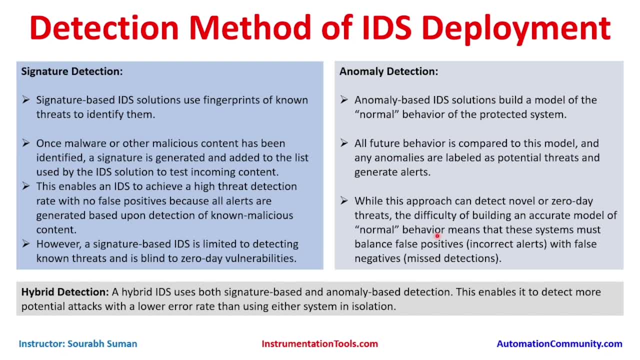 maturing and say enough, mature now. so maturing and say enough, mature now. so most of the ideas solutions. if you find most of the ideas solutions, if you find most of the ideas solutions, if you find they have a very good detection, they have a very good detection. 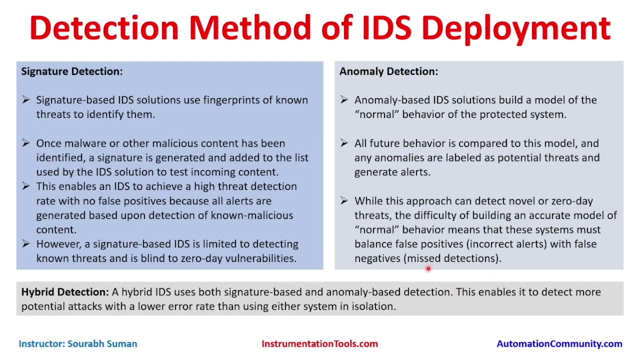 they have a very good detection capabilities and very less false capabilities and very less false capabilities and very less false negatives also. so these are the two negatives also. so these are the two negatives also. so these are the two types of signature and anomaly detection. types of signature and anomaly detection. 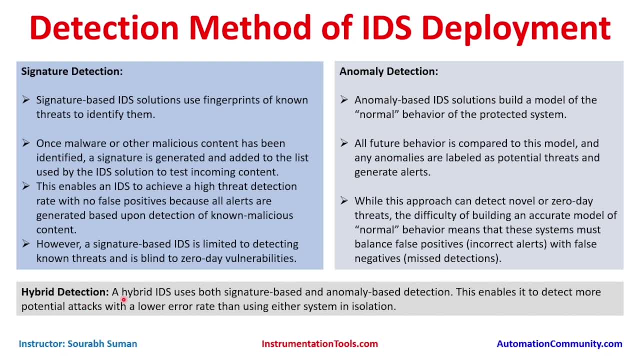 types of signature and anomaly detection. now there is one third type and this is now. there is one third type and this is now. there is one third type and this is quite good. it is hybrid ideas. uses both quite good. it is hybrid ideas. uses both quite good. it is hybrid ideas. uses both signature based as well as anomaly based. 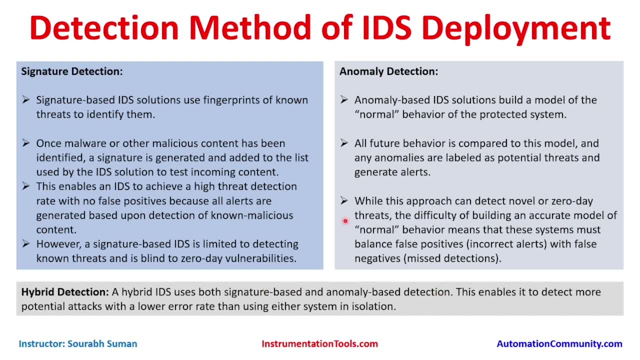 signature based as well as anomaly based. signature based as well as anomaly based detection. so it will work on this detection. so it will work on this detection. so it will work on this: signature based also, and then anomaly signature based also, and then anomaly signature based also, and then anomaly based also. so this enables it to detect. 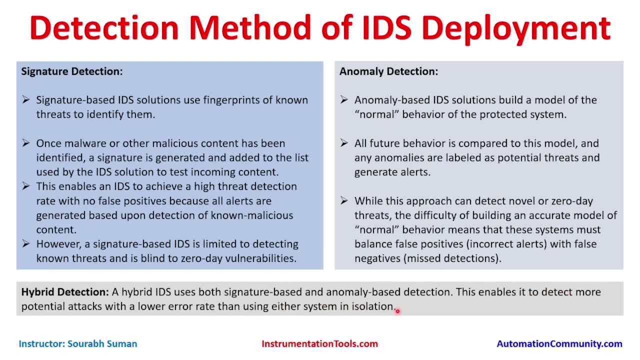 based also, so this enables it to detect. based also so this enables it to detect more potential attacks with lower error, more potential attacks with lower error, more potential attacks with lower error rate, and using either system in rate and using either system in rate and using either system in isolation also. 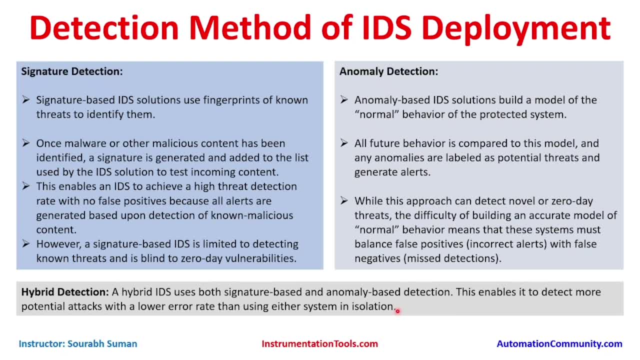 isolation also, isolation also, so, so so hybrid detection is recommended mode to hybrid detection is recommended mode to hybrid detection is recommended mode to implement in any environment. if your implement in any environment, if your implement in any environment, if your environment is really large, you should go. environment is really large, you should go. 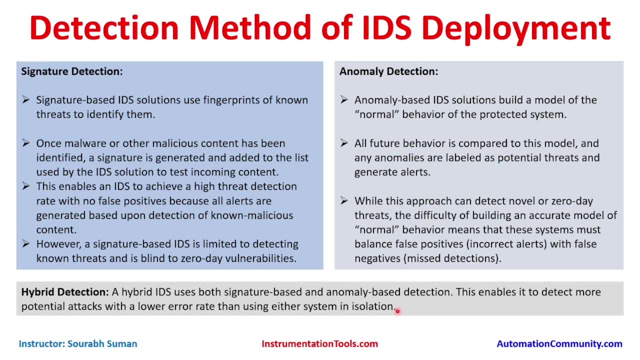 environment is really large. you should go for the hybrid detection tools, so that for the hybrid detection tools, so that for the hybrid detection tools, so that that will give you a like both. it will, that will give you a like both. it will, that will give you a like both. it will be in learning mode also, and then it. 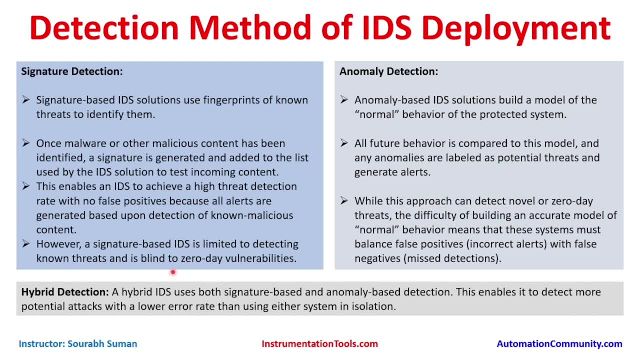 be in learning mode also, and then it be in learning mode also, and then it will be in detection mode due to the will be in detection mode due to the will be in detection mode due to the signature based detection capability as signature based detection capability, as signature based detection capability as well. 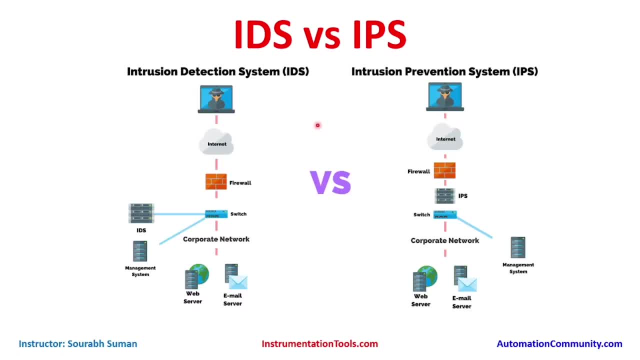 well, well, now moving ahead. let's see it's a basic, now moving ahead. let's see it's a basic. now moving ahead. let's see it's a basic thing that what is ids and what is the thing that, what is ids and what is the thing that, what is ids and what is the difference between ids and ips. 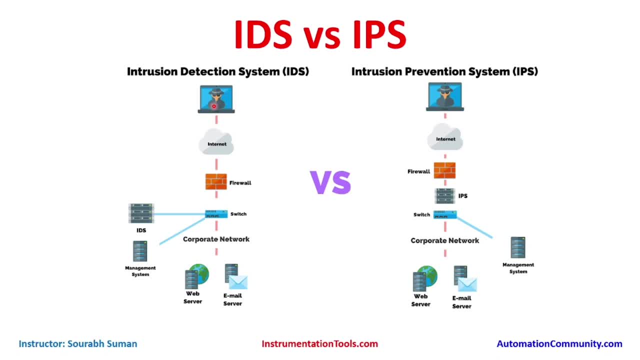 difference between ids and ips. difference between ids and ips. so how can we install our ids? so let's so. how can we install our ids? so let's so. how can we install our ids? so let's see, this is a malesis hacker or user. see, this is a malesis hacker or user. 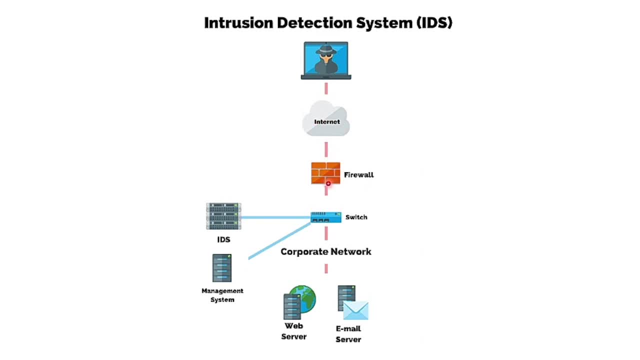 see, this is a malesis hacker or user, and this is the internet untrusted, and this is the internet untrusted, and this is the internet untrusted network. and then we have a firewall as a network, and then we have a firewall as a network, and then we have a firewall as a boundary protection device. then we have 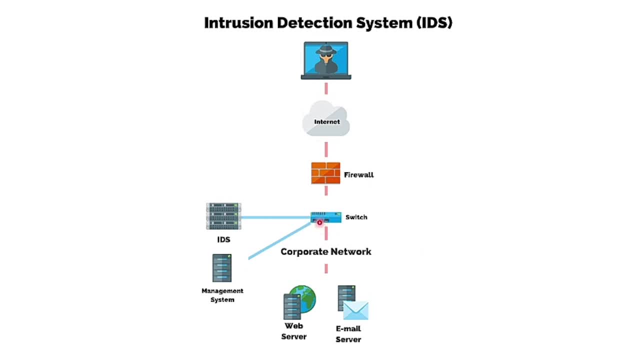 boundary protection device. then we have boundary protection device, then we have a switch, a switch, a switch. then what we will do, we will configure a. then what we will do, we will configure a. then what we will do, we will configure a mirror port on this switch and then 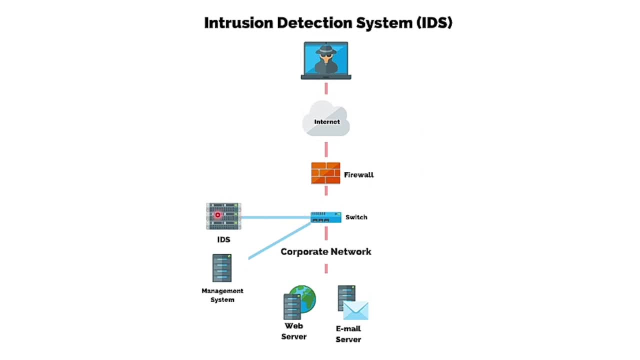 mirror port on this switch and then mirror port on this switch and then mirror or span port and then we'll feed mirror or span port and then we'll feed mirror or span port and then we'll feed that. that that mirror data to the ids. so ids will. 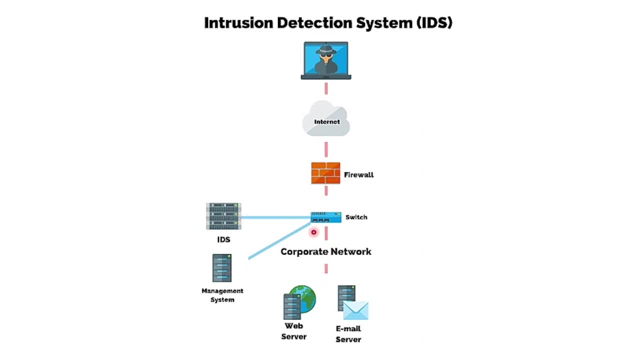 mirror data to the ids, so ids will mirror data to the ids, so ids will analyze all those traffic. whatever is analyze all those traffic, whatever is analyze all those traffic, whatever is passing through this switch, passing through this switch, passing through this switch, then management is also connected to this. 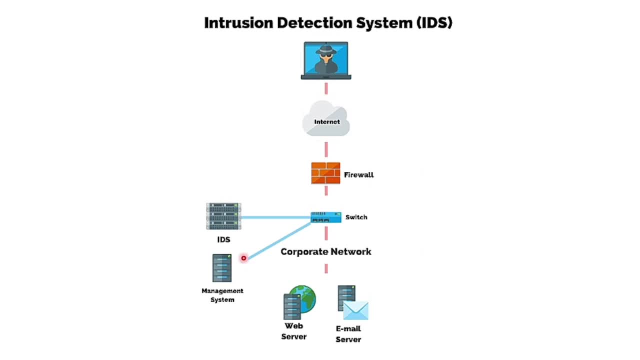 then management is also connected to this, then management is also connected to this and there is a corporate network, so, and there is a corporate network, so, and there is a corporate network. so this is the point where we can, this is the point where we can, this is the point where we can check all the traffic coming from. 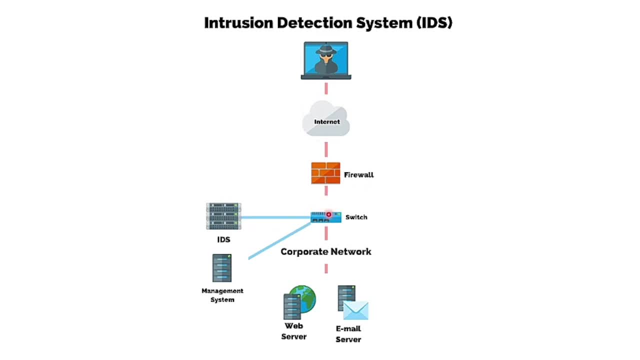 check all the traffic coming from. check all the traffic coming from understood network to our network. understood network to our network, understood network to our network. but it all the traffic, one copy will go. but it all the traffic, one copy will go. but it all the traffic, one copy will go to this ids. 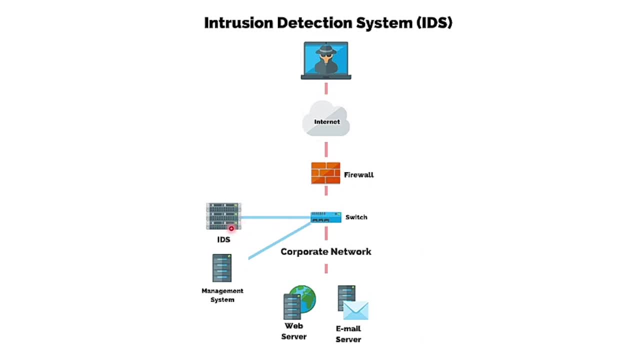 to this ids, to this ids. so here ids, you can see it is getting so, here, ids, you can see it is getting so here, ids, you can see it is getting only the span traffic. so even if a only the span traffic, so even if a only the span traffic, so even if a threat is detected, it will only create a. 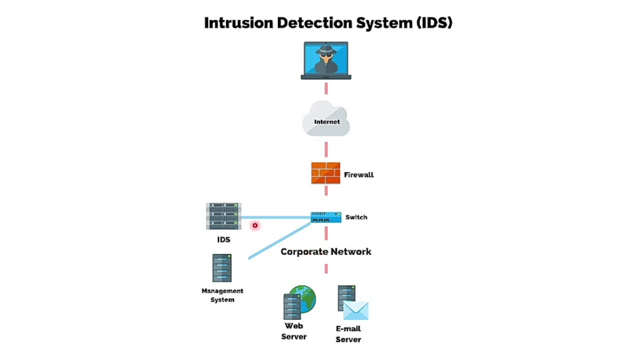 threat is detected, it will only create a threat is detected, it will only create a alert. it has nothing to do, it cannot alert. it has nothing to do. it cannot alert. it has nothing to do. it cannot prevent that to happen. so the ids is a. prevent that to happen, so the ids is a. 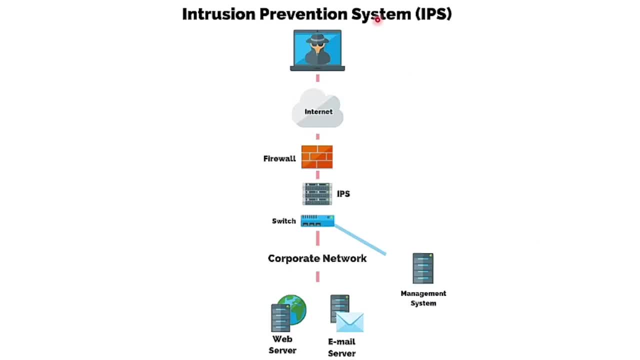 prevent that to happen. so the ids is a detection tool, basically detection tool, basically detection tool, basically now coming to the ips, now coming to the ips, now coming to the ips. it's the same network, similar network. it's the same network, similar network. it's the same network, similar network. we are putting ips in series. 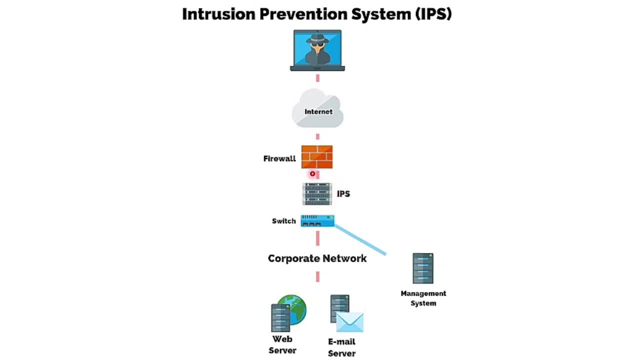 we are putting ips in series. we are putting ips in series. so after firewall there is a ips, so after firewall there is a ips, so after firewall there is a ips solution. some firewalls like next solution, some firewalls like next solution, some firewalls like next generation firewall, they have ips in. 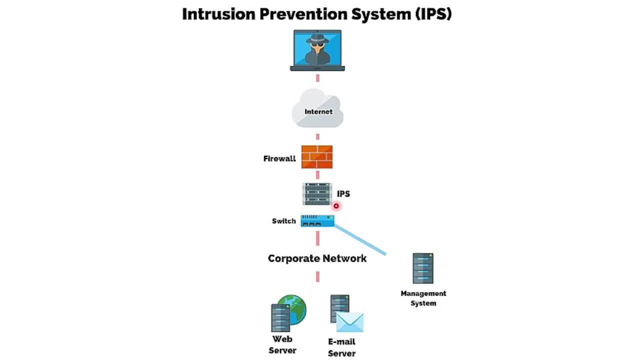 generation firewall. they have ips in generation firewall. they have ips in built with that, built with that, built with that. but you have option to keep that ips in. but you have option to keep that ips in. but you have option to keep that ips in a monitoring mode or in a protection. 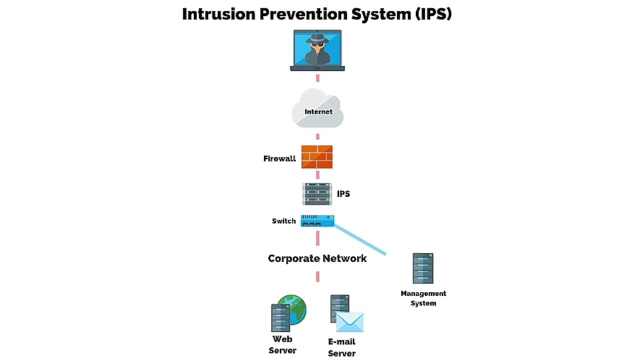 a monitoring mode or in a protection, a monitoring mode or in a protection mode. so if you keep that ips in a mode, so if you keep that ips in a mode, so if you keep that ips in a monitoring mode, it will become ids. monitoring mode: it will become ids. 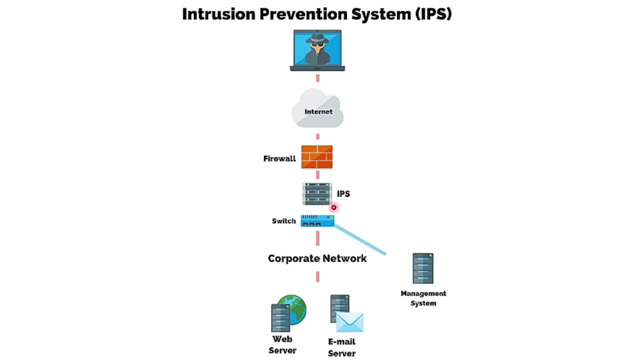 monitoring mode. it will become ids. if you keep that ips in a protection, if you keep that ips in a protection, if you keep that ips in a protection mode, it will, it will become protection mode. it will, it will become protection mode. it will, it will become protection. so what will happen here? so, if something, 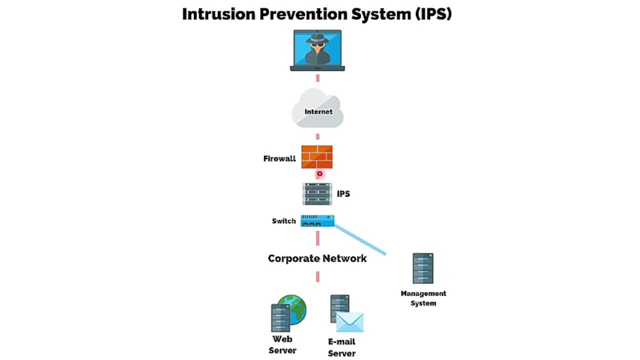 so what will happen here? so if something? so what will happen here? so if something comes out here, comes out here, comes out here some threat or malware? it identifies it. some threat or malware. it identifies it. some threat or malware. it identifies it will block that traffic to go downwards. 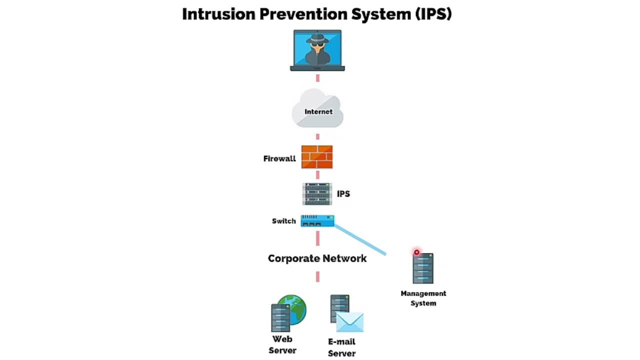 will block that traffic to go downwards, will block that traffic to go downwards. so it will prevent that threat to. so it will prevent that threat to, so it will prevent that threat to further propagate into this network, further propagate into this network, further propagate into this network. so ips is quite. 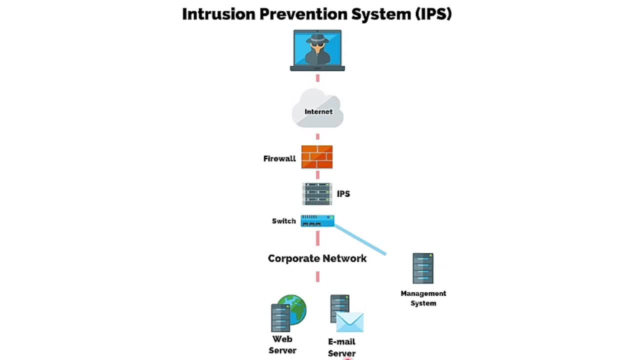 so ips is quite so. ips is quite good, good. good for the systems where there is no any, for the systems where there is no any, for the systems where there is no any down down, down time in case of blockage of the traffic. so time in case of blockage of the traffic. so. 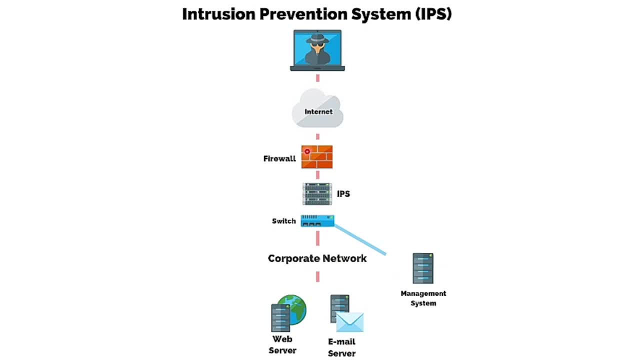 time in case of blockage of the traffic. so let us suppose if this is your, let us suppose if this is your, let us suppose if this is your industrial network, industrial network, industrial network, and you have implemented a ips, and you have implemented a ips and you have implemented a ips. in case of the false negatives, this: 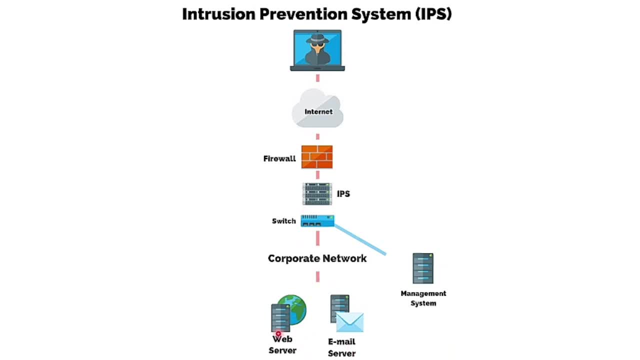 in case of the false negatives, this, in case of the false negatives, this, this communication will break and there this communication will break and there this communication will break and there might be performance, might be performance, might be performance. issues in your industrial network. because issues in your industrial network, because 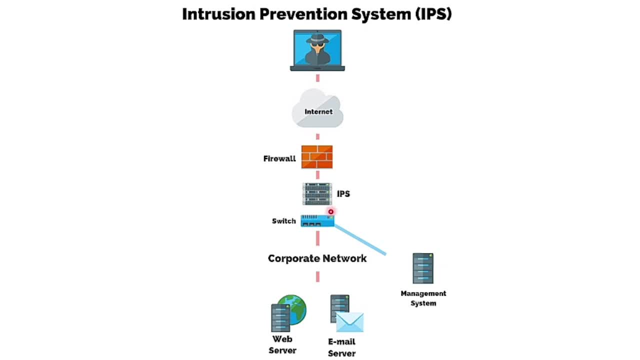 issues in your industrial network, because that was a false negative. that was a false negative. that was a false negative, like that was not actual alarm. that was like that was not actual alarm. that was like that was not actual alarm. that was just like, just like, just like. this system is not matured enough to 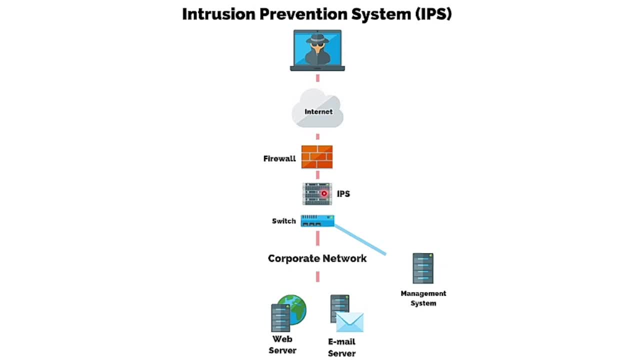 this system is not matured enough to. this system is not matured enough to detect, whether, detect, whether detect whether it was a false, negative or false. it was a false, negative or false positive, positive, positive. so in those cases it is recommended to. so, in those cases it is recommended to. 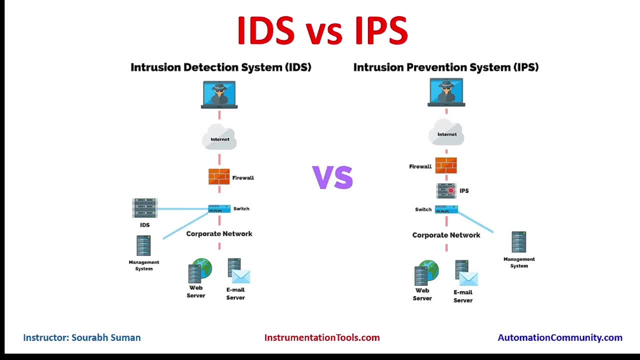 so in those cases it is recommended to install a ips in a monitoring mode, install a ips in a monitoring mode, install a ips in a monitoring mode, in a detection mode, and once in a detection mode, and once in a detection mode, and once your system gets matured it has good 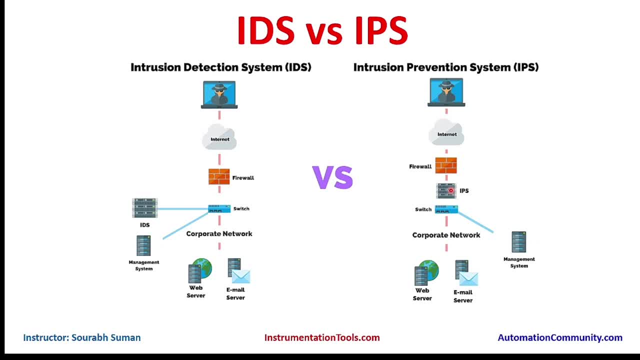 your system gets matured, it has good. your system gets matured, it has good learning, then you can switch it back to learning, then you can switch it back to learning, then you can switch it back to the protection mode, the protection mode, the protection mode. so that is one basic implementation of 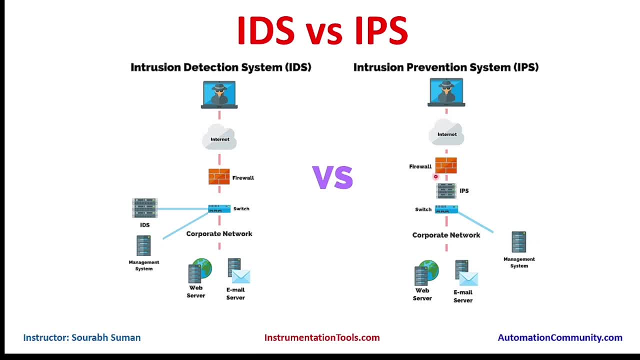 so that is one basic implementation of. so that is one basic implementation of ips, ips, ips. now hope you have understood difference now hope you have understood difference. now hope you have understood difference between between ips and ids. similarly ips and ids. similarly ips and ids. similarly, uh, you can create it on a. you can put. 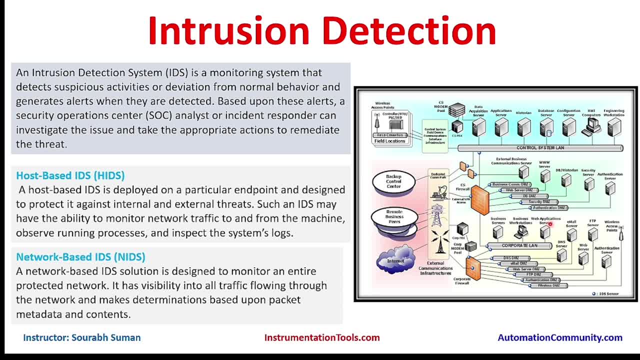 uh, you can create it on a, you can put. uh, you can create it on a, you can put it on a big network also. it on a big network also. it on a big network also. like we saw here, now we have multiple ids. like we saw here, now we have multiple ids. 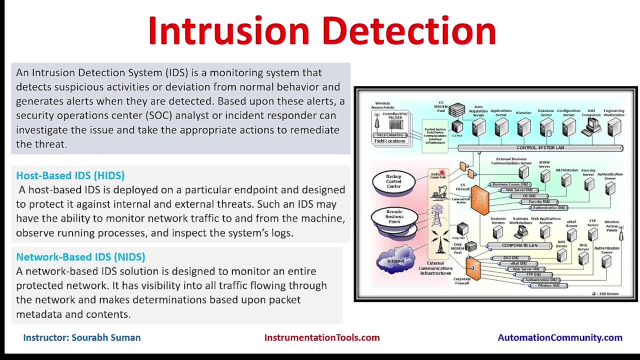 like we saw here. now we have multiple ids sensors and all these ids sensors will sensors and all these ids sensors will sensors and all these ids sensors will be connected to a, be connected to a. be connected to a central console where you can see all central console where you can see all. 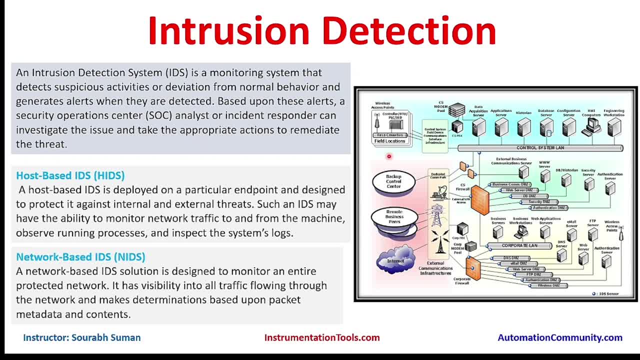 central console where you can see all the alerts from everywhere. it is not the alerts from everywhere, it is not the alerts from everywhere. it is not like distributed, so ids consists of like distributed, so ids consists of like distributed, so ids consists of, basically, sensors. it will have sensors. 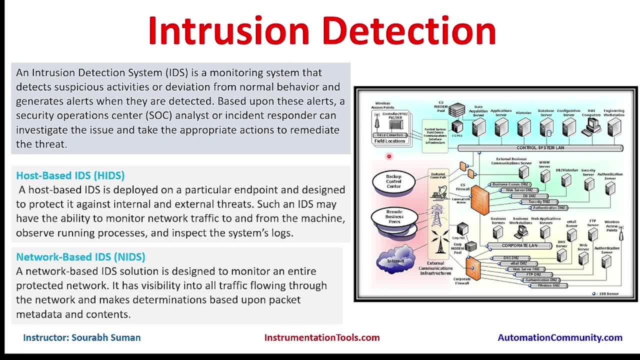 basically sensors. it will have sensors, basically sensors. it will have sensors. it will have a. it will have a. it will have a central uh com computing module. it will central uh com computing module. it will central uh com computing module. it will have a thread engine. it will have.